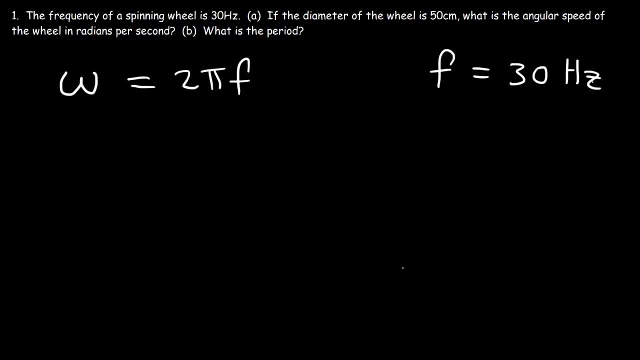 And the frequency represents the number of cycles that occur per unit time. So in this case the cycles are rotations or revolutions. So if the frequency is 30 Hz, that means that the wheel makes 30 revolutions every second. Now, when you think of 2 pi, what do you think of? 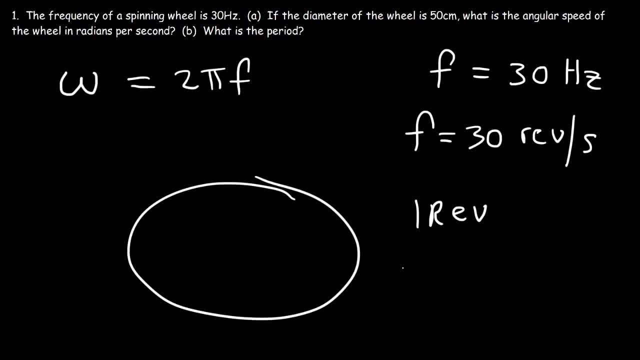 One revolution around a circle is equal to 360 degrees, And 360 degrees is 2 pi radians, Because 180 is equal to pi, So one revolution around a circle is 2 pi radians, So omega is equal to 2 pi radians per revolution. 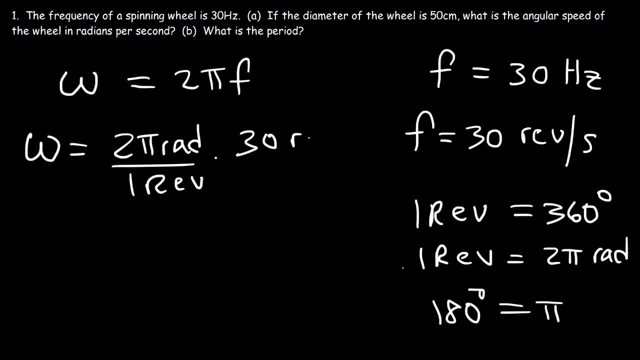 Multiplied by the frequency, which is 30 revolutions per second. So notice that the unit revolutions cancel. I want to set it up in such a way so you can see how frequency can give you the angular speed in radians per second. So in this example it's 2 pi times 30.. 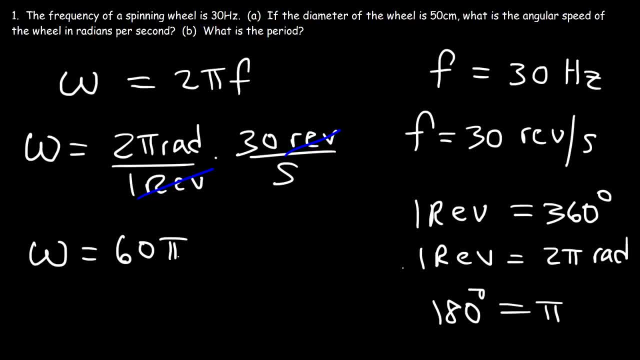 So omega is going to be 60 pi radians per second. Now, if you want to get the decimal value of that, this is going to be 188.5 radians per second. So that's the angular speed in this problem. Now let's move on to part B. 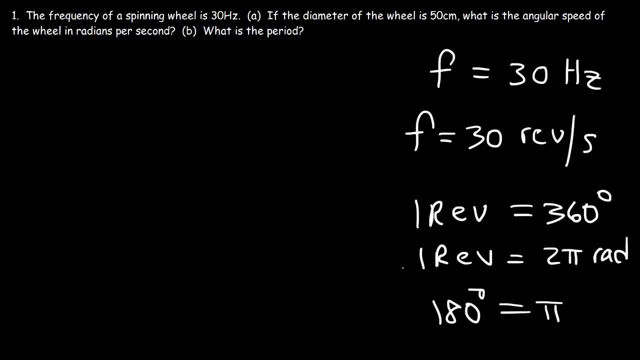 What is the period? The period is the time divided by the number of cycles that occurs. So if we have 30 cycles that occur in one second, then the period is one second per 30 cycles, In this case, 30 revolutions. 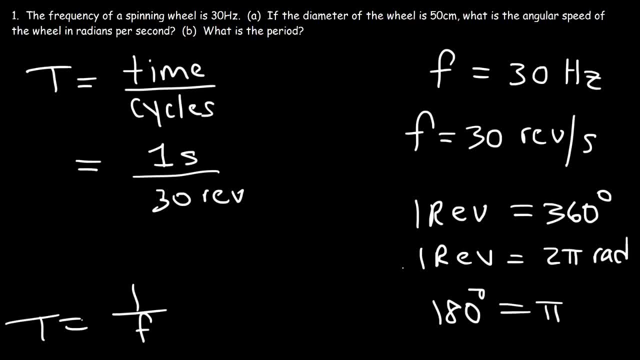 So period is simply 1 over f. It's the reciprocal of the frequency. So 1 divided by 30 is 0.033 seconds. So what that means is that the wheel makes 1, 1 revolution in 0.033 seconds. 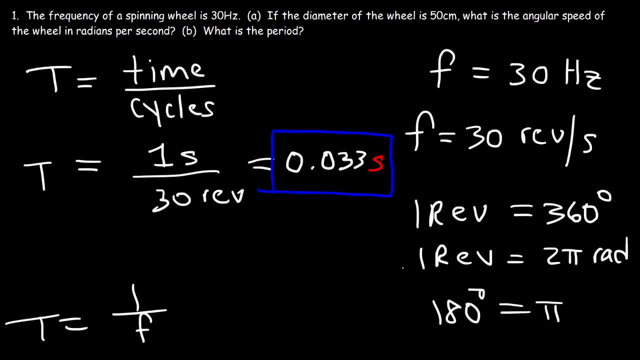 So the period tells you the time it takes to make 1 revolution or 1 complete cycle around the circle, Whereas the frequency tells you the number of cycles that can be made in 1 second. So in 1 second the wheel is going to spin 30 times. 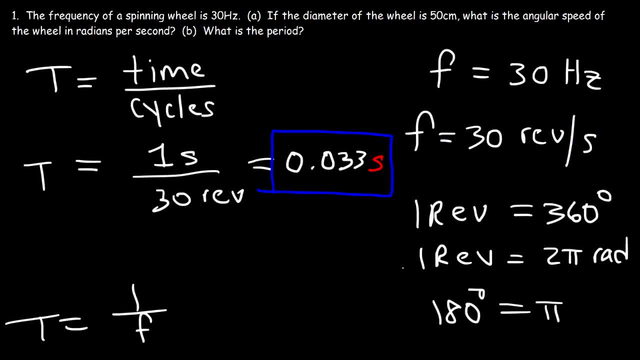 That's the frequency, And the period tells you that the wheel will spin once every 0.033 seconds. So that's the frequency, And the period tells you that the wheel will spin once every 0.033 seconds. So hopefully this clarifies the definition between period and frequency. 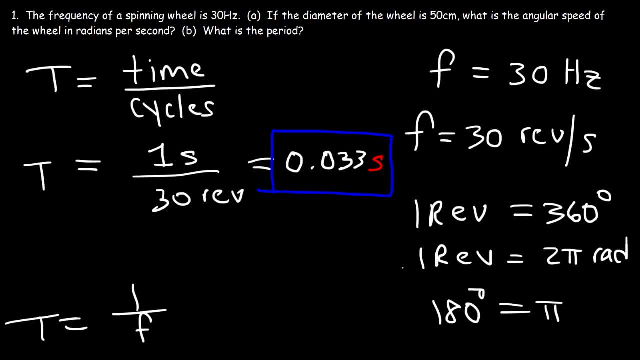 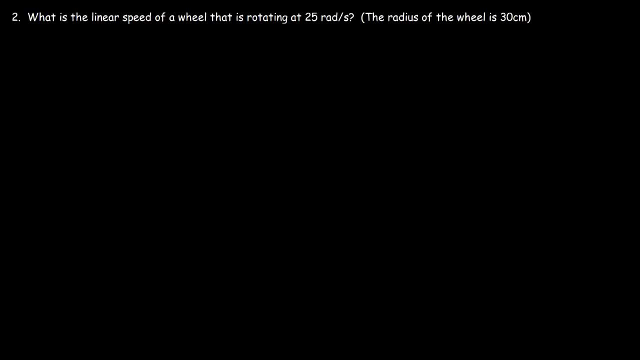 So frequency tells you how many cycles will occur in 1 second and the period tells you how long it takes just to make 1 cycle. Number two: What is the linear speed of a wheel that is rotating that 25 radians per second? 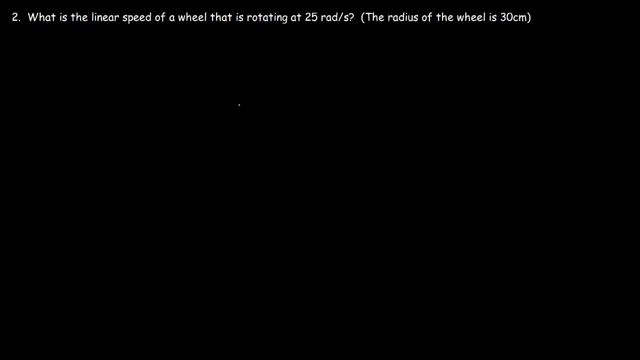 And we're given the radius of the wheel. It's 30 centimeters. So how can we find the linear speed of the wheel, given its rotational speed of 25 radius per second? So what should we do? The equation that we need is this: equation: V is equal to omega times R. 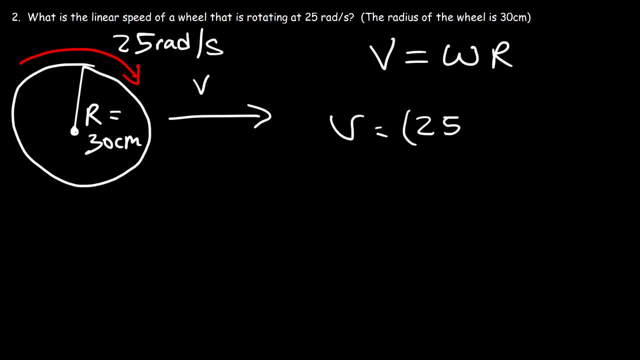 So all it is is just omega, which is 25, multiplied by the radius of the wheel. but we need that in meters. So to convert 30 centimeters into meters, divide it by 100, 30 divided by 100 is 0.30. 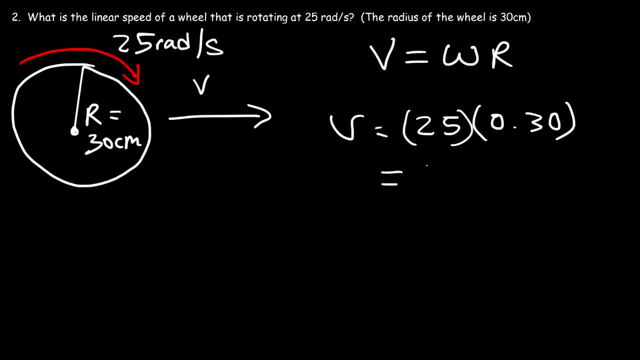 So 25 times 0.3 is 7.5. So the linear speed is 7.5 meters per second. Now let's make sense of the units. So omega was in radians per second, And the radius. I like to think of it like this: 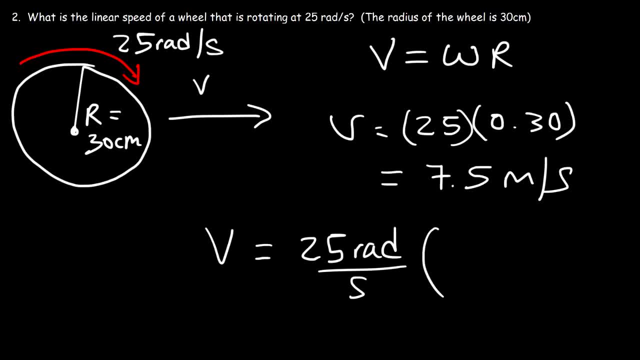 I like to think of it as the length per radian, So the radius is 0.3 meters, but it's really 0.3 meters per radian, And so this will give you 7.5 meters per second. Now for those of you who want to know why I like to think of the radius as being the 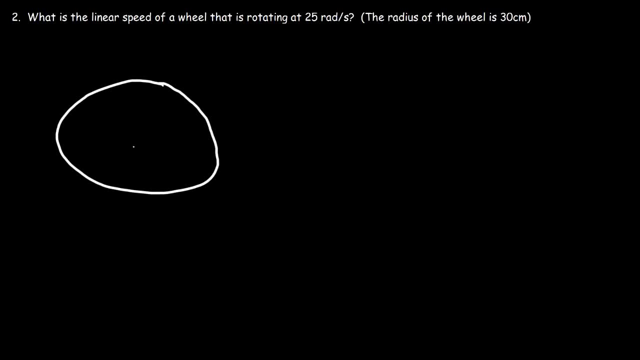 length per radian. Here's why. Let's say, if we draw an arc, So this is going to be S, the arc length, And this is the angle, theta, And this is the radius of the circle. The arc length is equal to the angle in radians times the radius of the circle. 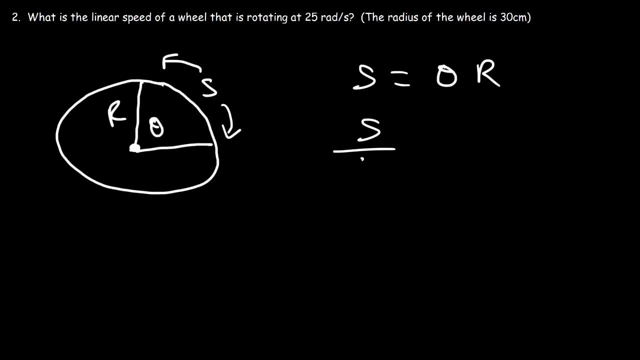 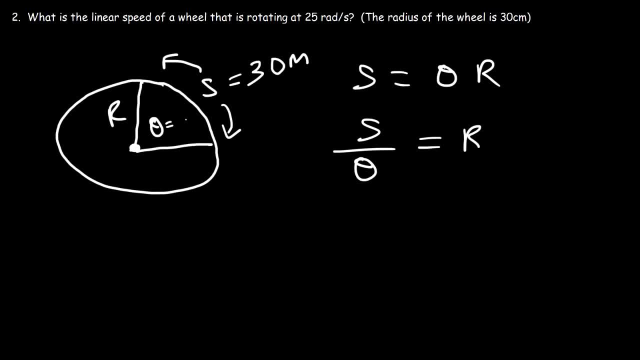 So let's say, if we have an arc length. So let's say, if we have an arc length of 30 meters And let's say the angle is 2 radians, So it's going to be 30 meters per 2 radians. 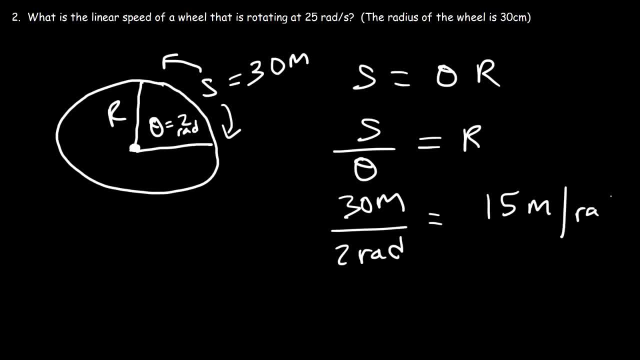 So the radius will be 15 meters per radian. So what does this mean? This is the arc length when the angle is 1 radian. So when the angle was 2 radians, the arc length was 30 meters. now, if you reduce the angle to 1 radian, the arc 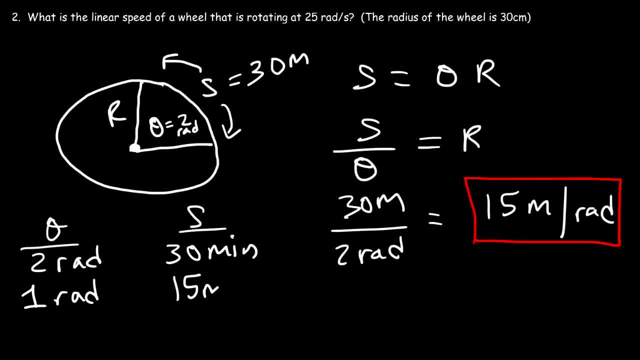 length will be equal to the radius, which is 15 meters. I wrote minutes for some reason, but let's correct that, so that's why I like to think of the radius as being the arc left when the angle is 1 radian, so I think of it as meters per. 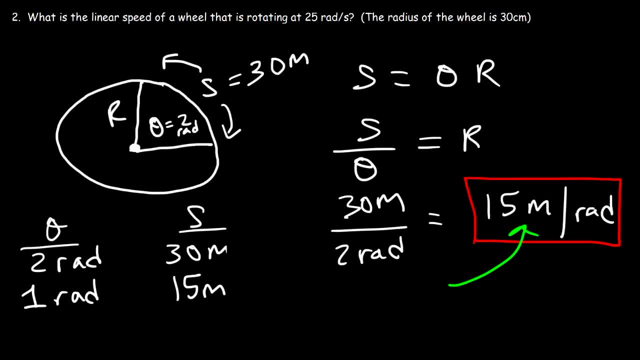 radian. so all of this leads me to the conclusion that 1 radian is equal to the length of the radius. so when the angle is 1 radian, the arc length of the circle is equal to the length of the radius of the circle, which in this example is 15. 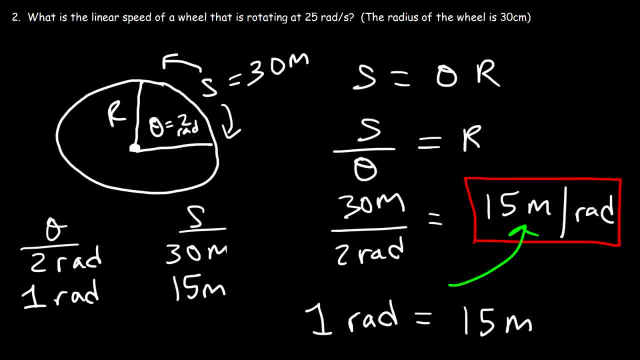 meters. so this is useful for conversions. let's say if I want to convert linear speed from radians per second to rotations per minute or revolutions per minute. so knowing the conversion factor between radians and meters is very useful. and it's equal to the radius of the circle. so let's say if the radius of the circle 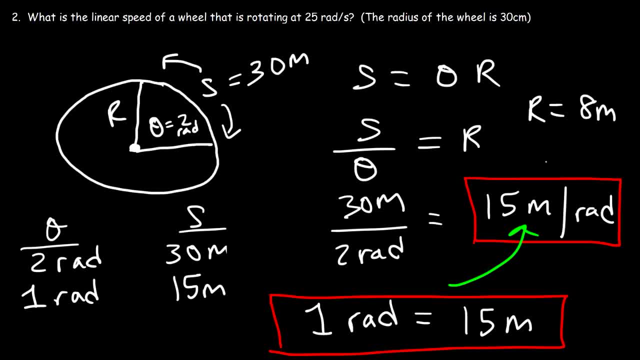 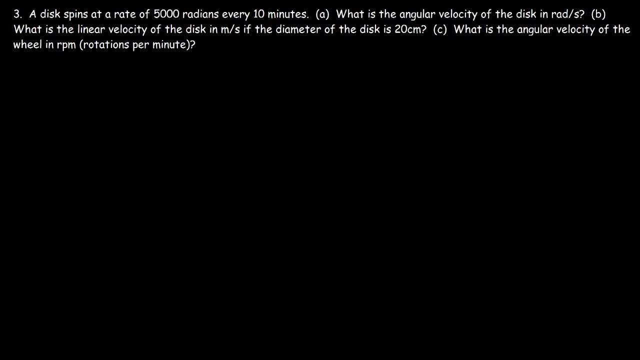 is 8 meters. I can come up with this conversion: 1 radian represents an arc length of 8 meters if the radius is 8 meters, so the radius would be 8 meters per radian. let's work on number three. a disc spins at a rate of 5,000. 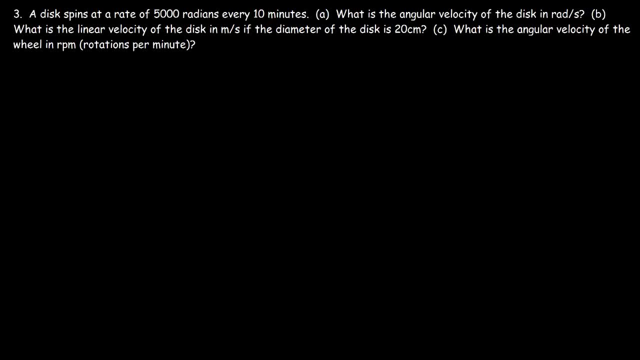 radians every 10 minutes. what is the angular velocity of the disc in radians per second? so to calculate the angle of velocity we can use this equation: it's the angular displacement divided by the change in time. the angular displacement is the amount that the disc spins in radians, so it spins a distance of. 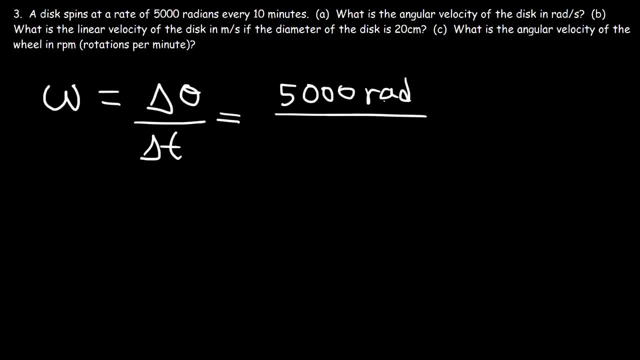 5,000 radians and we have the time, which is 10 minutes, but we'll need that. in seconds. now, one minute is equal to 60 seconds, which means that 10 minutes is 60 times 10 or 600 seconds. so the disc spins 5,000 radians every 600 seconds. so 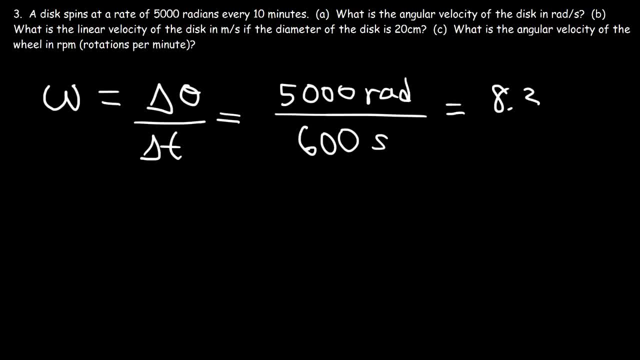 therefore, the angular velocity is 8.33 radians per second. so that's it for part a. now let's move on to part B. what is the linear velocity of the disc in meters per second if the diameter of the disc is 20 centimeters? so we're given the 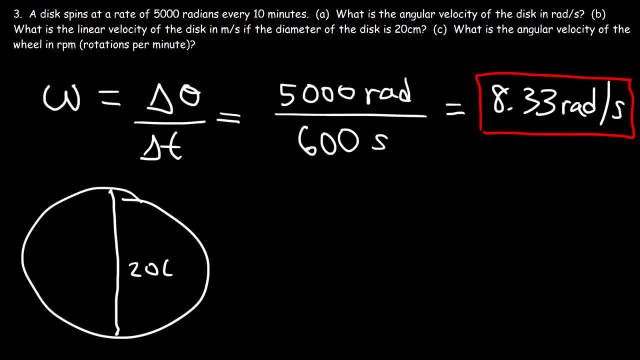 diameter of the disc is 20 centimeters. now we need to use that to find the radius. the radius of the disc has to be half of the diameter, so it's 10 centimeters. so we get say the radius is 10 centimeters per radian, so that means the length of one. 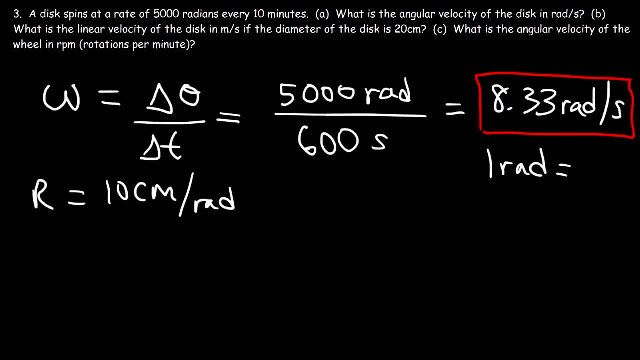 radian, or one radian has an arc length of 10 centimeters, but we need to convert centimeters into meters, so we got to divide that by 100, so that's 0.1 meters per radian. so now let's calculate the linear velocity. so V is equal to Omega. 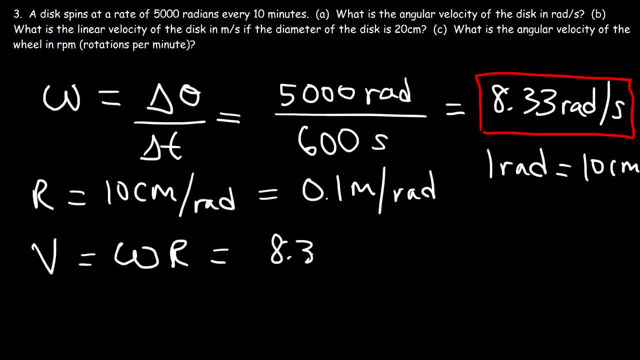 times R. Omega is 8.33 radians per second and the radius is 0.1 meters per radian. so the arc length is 0.1 meters when the angle is 1 radian. so these two will cancel and then we'll have the units in meters per second, so 8.33 times. 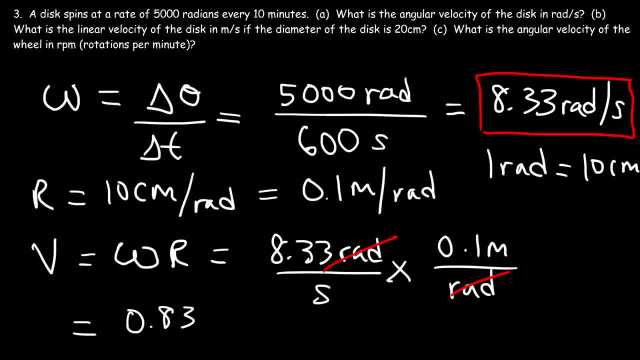 0.1 is simply 0.833 meters per second. so this is the answer to Part B. now let's move on to Part C. what is the angular velocity of the wheel in rotations per minute, which is equivalent to revolutions per minute? so how can we find that answer? 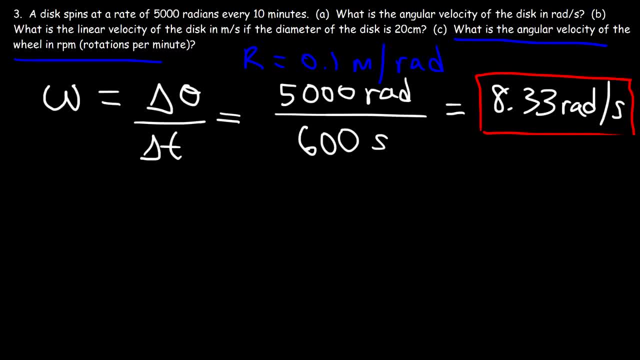 so all we got to do is convert the angular velocity from radians per second to rotations per minute, or simply revolutions per minute. so how can we go about doing that? well, let's start with what we have: 8.33 radians per second. now we can convert seconds into minutes. 60 seconds is equal to one minute. 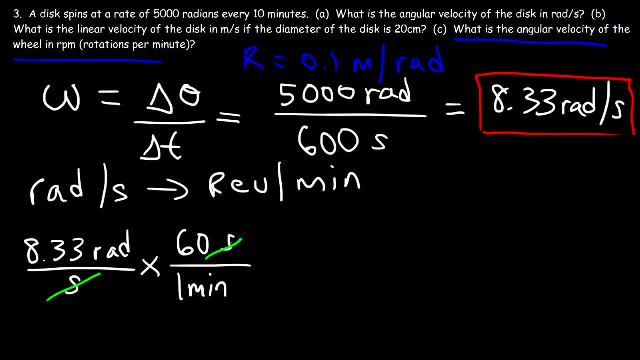 so the unit seconds cancel. next we can convert radians to revolutions, so it's 2 pi radians per revolution, but I need to put radians on the bottom, so one revolution is equal to 2 pi radians, and so now we have the unit revolutions per minute, which is basically RPMs. so it's eight point thirty three times 60. 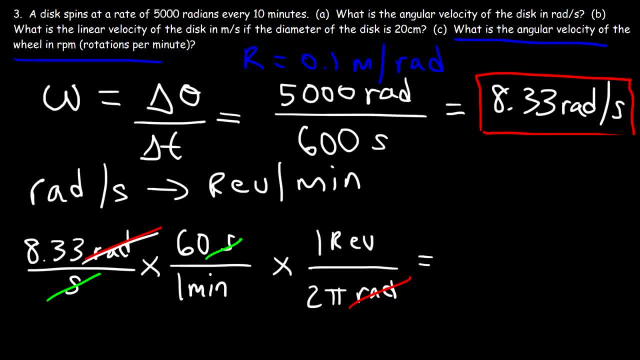 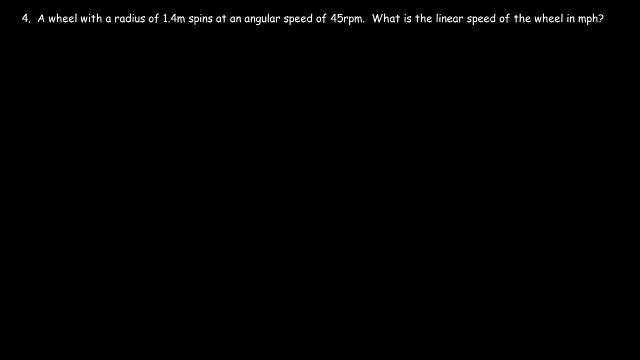 divided by 2 pi, and so this is going to be 79.5 rotations per minute. that's the answer. so here's the last question for this video. a wheel with a radius of one point four meters spins at an angular speed of 45 rotations per minute, or revolutions per 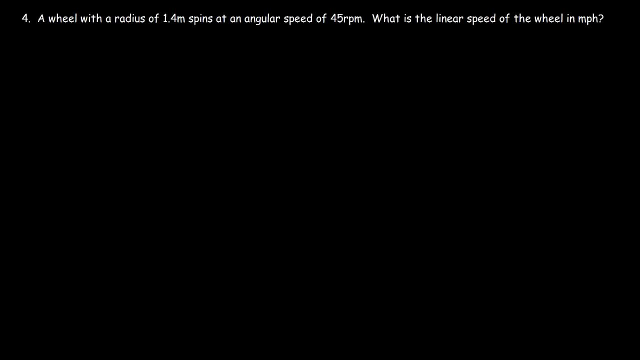 minute. What is the linear speed of the wheel in miles per hour? Go ahead and try this problem. So let's convert it from revolutions per minute to miles per hour. So we have 45 revolutions per minute. Now we need to convert minutes to hours: 60.